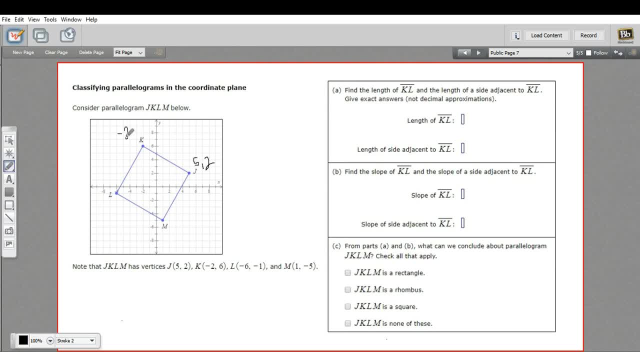 So j is 5, 2.. k is negative 2, 6. And l is negative 6, negative 1.. And m is 1, negative 5.. Okay, Our job here is to figure out what kind of a quadrilateral this is. 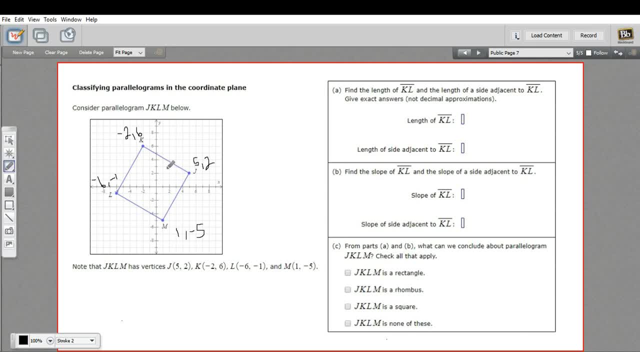 It sort of looks like a square, but we don't know for sure. We could know if we knew that all the side lengths were the same and if we knew what the angles were in here. So we're going to do some calculations to try to figure out side lengths. 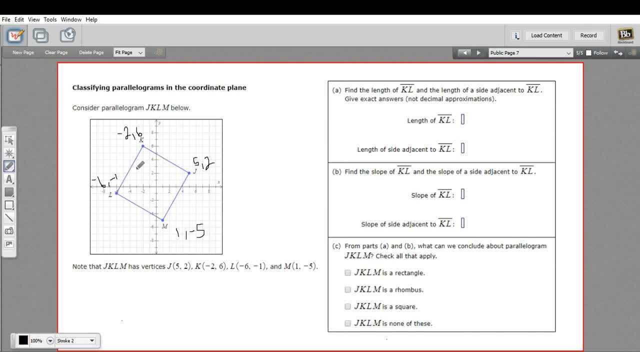 to try to figure out what angle these lines might be intersecting each other at. And in this problem they kind of walk you through. So they ask you to find the line. They ask you to find the length of kl first. So kl, this side right here. how do we find the length of that side? 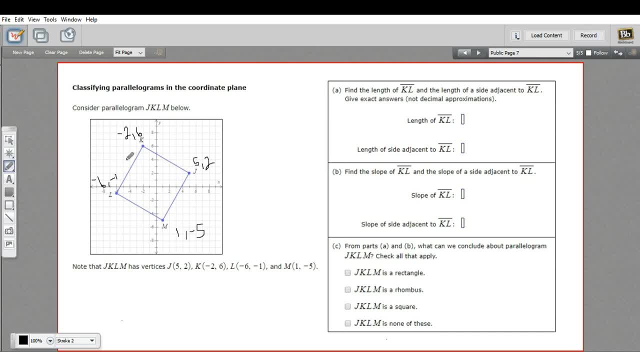 Well, since this is plotted in the coordinate plane, we can just calculate the distance between these two points, k and l, And to do that we'll use the distance formula, our old friend. And remember, the distance formula is the square root of the difference of the x-coordinate squared plus the difference of the y-coordinate squared. 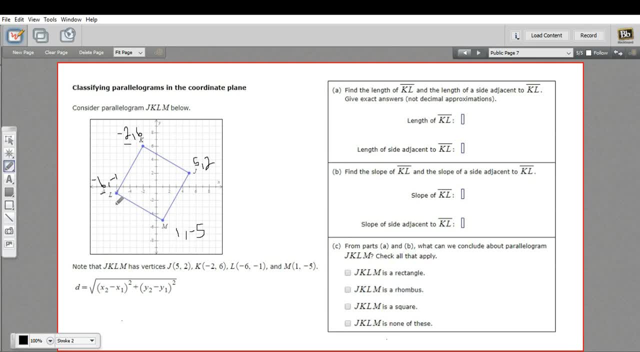 So let's look at the x-coordinates. We've got negative 2 and negative 6.. That's four spaces apart. So this is 4 squared plus and the y 6 to negative 1, that's 7 apart. so 7 squared. 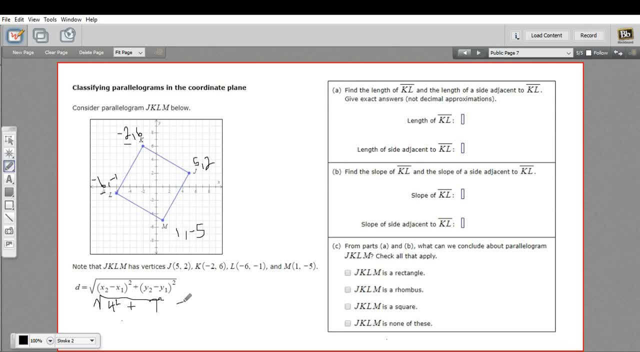 So this is the square root of 16 plus 49.. That is the square root of 65.. Okay, Then it says length of a side adjacent to kl. So it could be lm. It could be jk. I think I'm going to do jk. 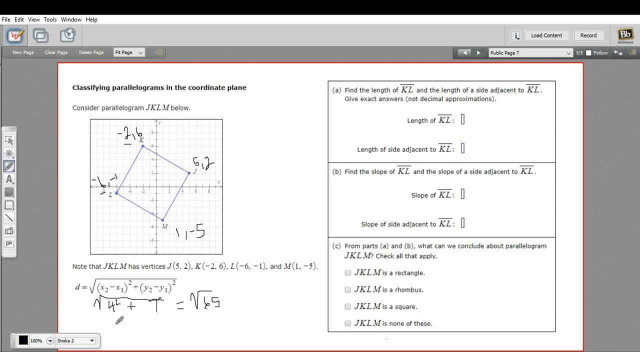 The x-coordinates negative 2 to 5, that's a change of 7.. So we've got 7 squared and the y-coordinate 6 to 2, that's a change in 4.. Oh, look at this. 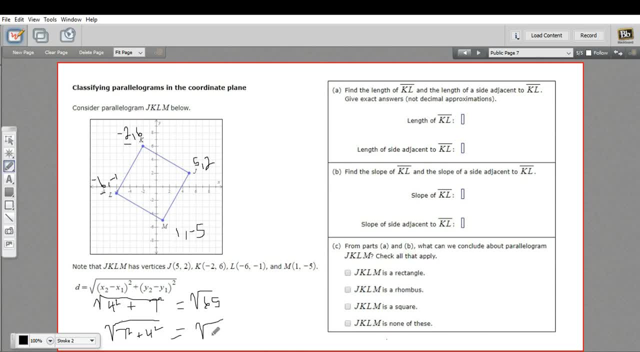 We have exactly the same thing. So this is also the square root of 65. So this side and this side are the same. The next thing they're asking us to do here is to find the slope of kl and the slope of a side that's adjacent.